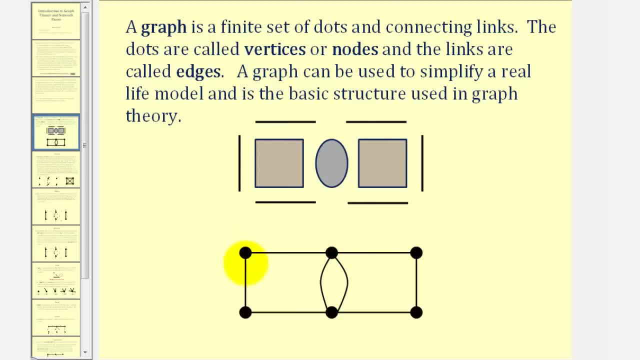 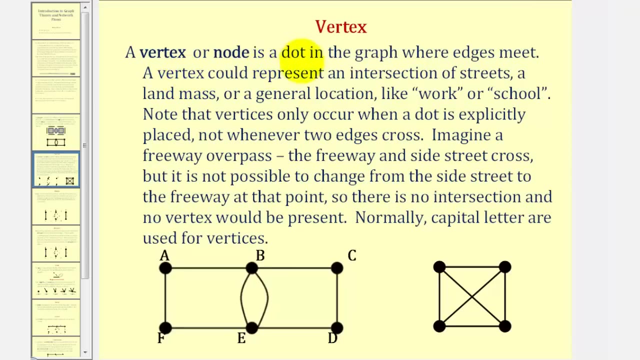 Notice how each intersection would be a dot, which we call a vertex, and each street would be an edge in the graph. Notice how here we have six vertices and eight edges. So again, a vertex or node is a dot in a graph where edges meet. 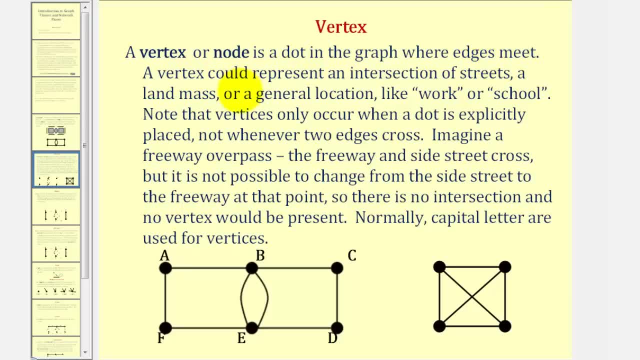 A vertex could represent an intersection of streets, a land mass or a general location like work or school. Note that vertices only occur where a dot is explicitly placed, not wherever two edges cross. Looking at this graph here, notice how we have two edges that cross, but because there's no dot. 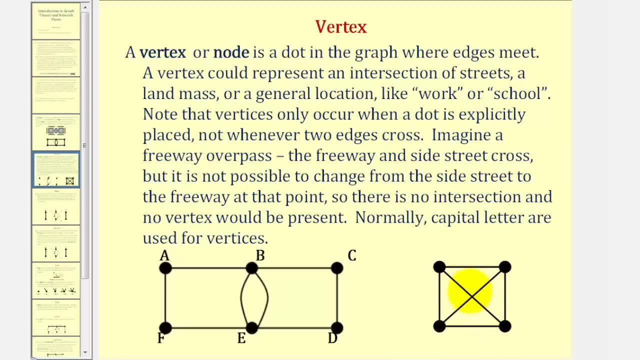 there's no vertex here. As a result, we can see that the dot is placed on the intersection of the street. So, as an example, imagine a freeway overpass The freeway and the side streets cross, but it is not possible to change from the side street. 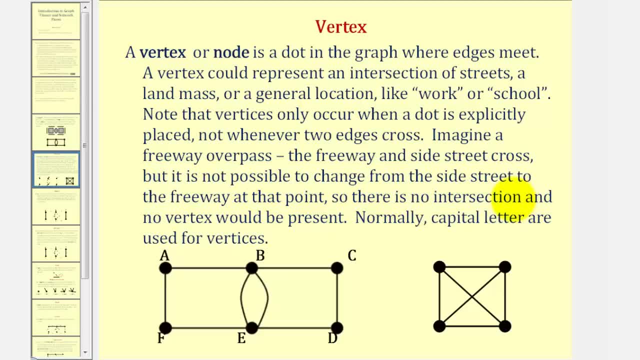 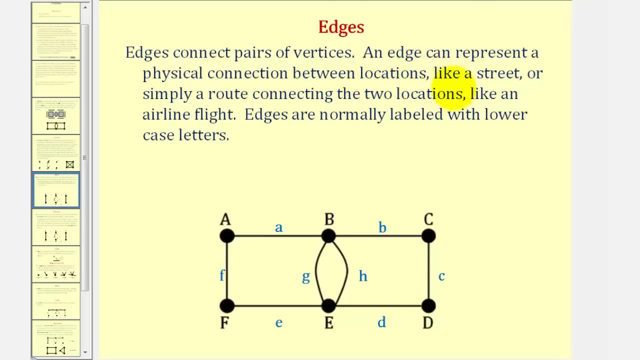 to the freeway at that point. so there's no intersection and no vertex would be present. Normally we use capital letters for the vertices. as we see here, Edges connect pairs of vertices. An edge can represent a physical connection between locations, like a street. 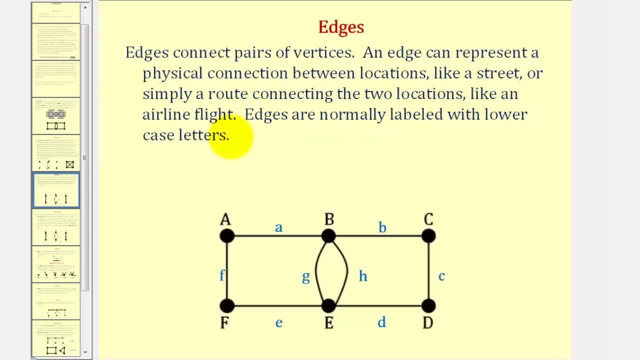 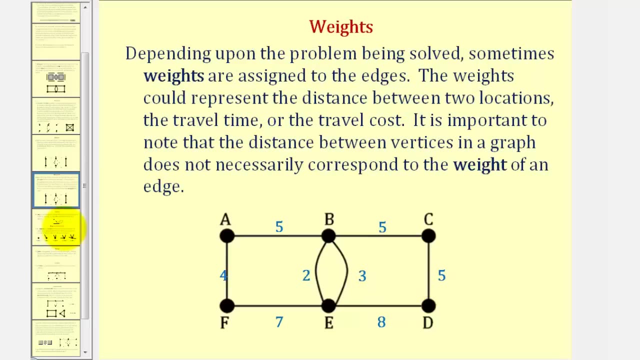 or simply a route connecting the two locations. like an airline flight Edges are normally labeled with lowercase letters, as we see here in blue. So again, we use capital letters for the vertices and lowercase letters for the edges normally Now, depending on the problem being solved. 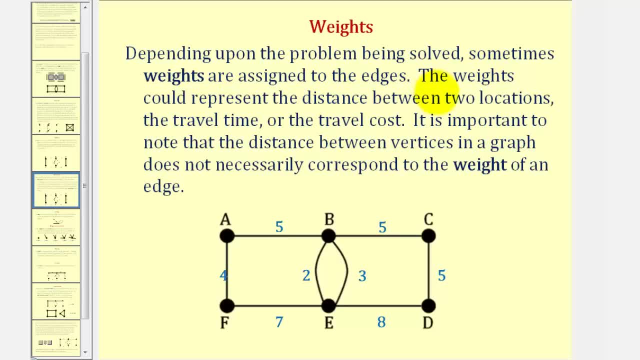 sometimes weights are assigned to the edges. The weights could represent the distance between two locations, the travel time or the travel cost, or several other possibilities. It is important to note that the number of edges and the distance between the vertices in a graph. 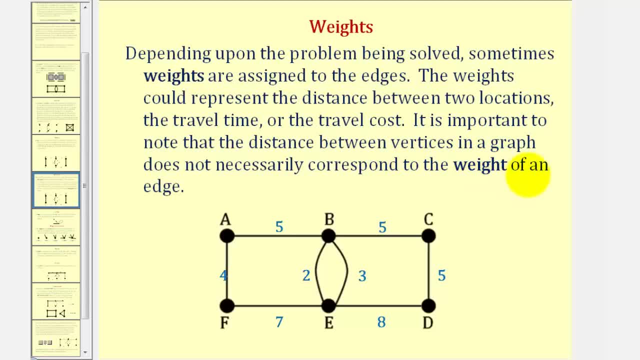 does not necessarily correspond to the weight of an edge. So looking at our graph here, notice how edge AF and edge CD are the same length but their weights are different. So graphs do not have to be drawn to scale. so it's important that we pay attention. 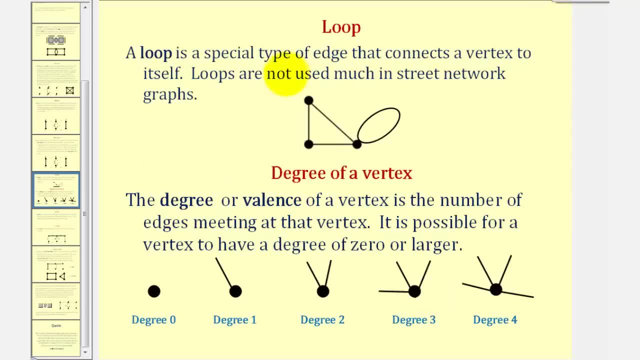 to the weights of the edges when they're given. A loop is a special type of edge that connects a vertex to itself. So, looking at this graph here, this would be a loop from this vertex. Now, the degree or valence of a vertex. 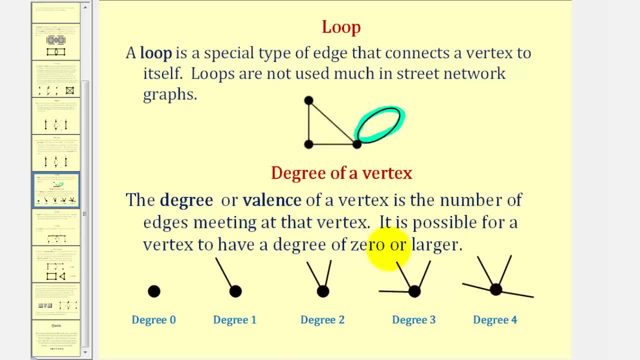 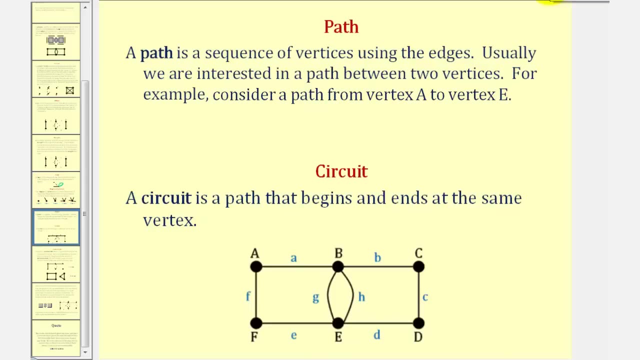 is the number of edges meeting at that vertex. It is possible for a vertex to have a degree of zero or larger. So here are several examples. Here's a vertex with degree zero, degree one, degree two, degree three and degree four. 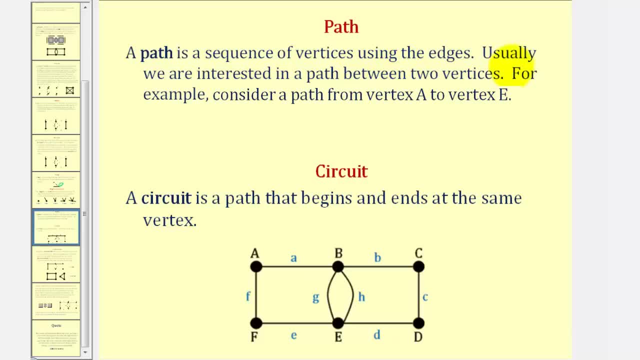 A path is a sequence of edges and a sequence of vertices. using edges, Usually we are interested in a path between two vertices, For example a path from vertex A to vertex E. So one possible path from vertex A to vertex E might look something like this: 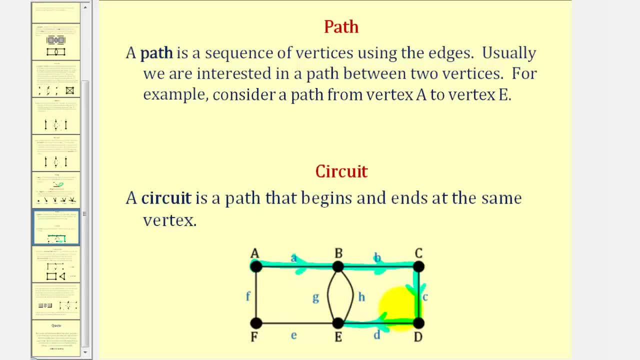 But of course there are several other paths, from vertex A to vertex E, For example. this would be another path from vertex A to vertex E, And of course there are others. A circuit is a path that begins and ends at the same vertex. 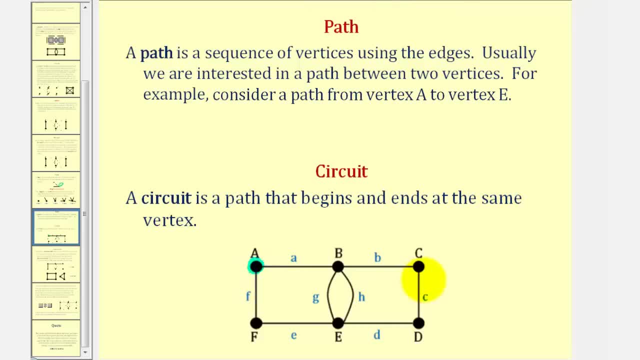 So, starting at vertex A, we can form several circuits. For example, we could go from vertex A to vertex B, to C, to D, to E, to F and then back to A. Another circuit might be from A to B to E. 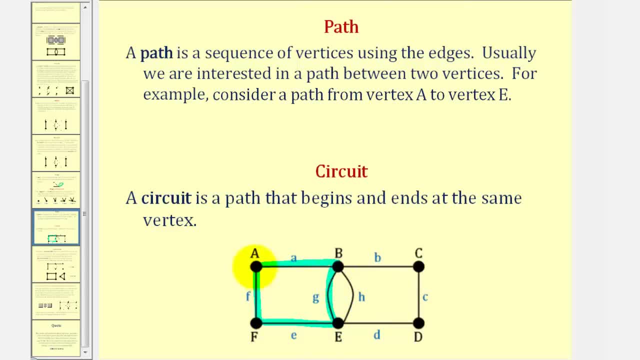 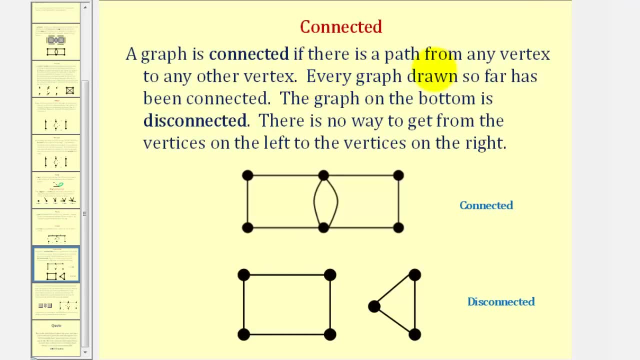 to F. back to A. This is another circuit containing vertex A. A graph is connected if there is a path from any vertex to any other vertex. So this first graph here is connected, because if we start at any vertex, let's say this vertex here. 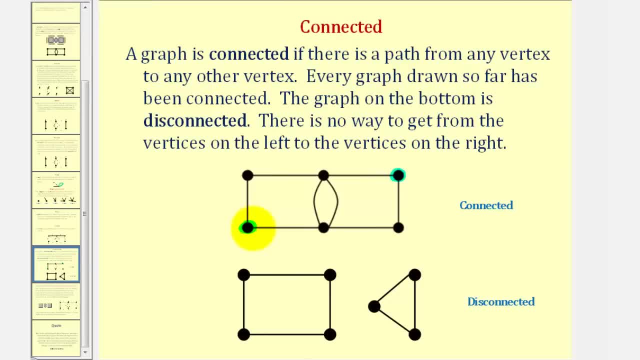 and then we select another vertex. let's say, this vertex- here it will always be- would be a path from this vertex to this vertex or any other two vertices we decide to select. One possible path would just be like this: But the graph on the bottom here is disconnected. 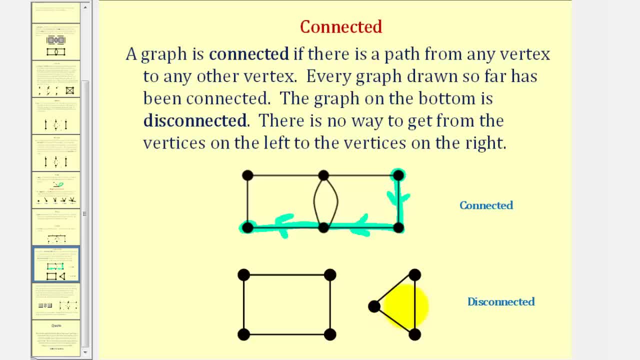 because there's no way to get from the vertices on the left to the vertices on the right, meaning there's no path from, let's say, this vertex to this vertex, because this graph is disconnected. So, to finish, let's go back to our opening example.